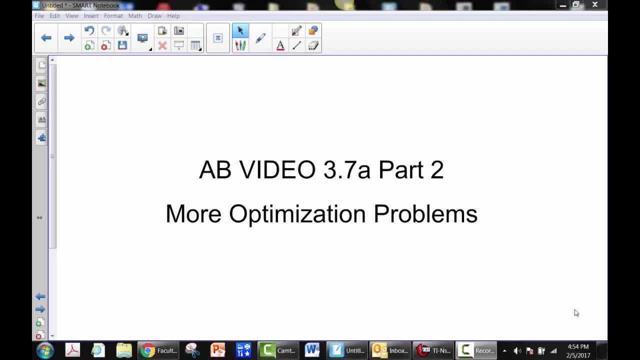 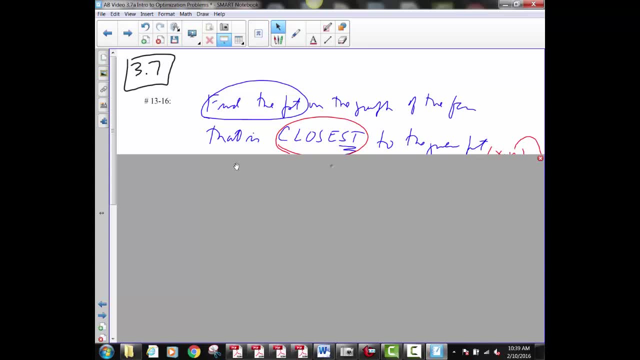 Hello, welcome to AB Video 3.7a, Part 2, More Optimization Problems. To be able to find the derivative of the critical numbers and find the relative maxes and mins. Okay, this one's a little complicated. Find the point on the graph of the function that is closest to the given point. 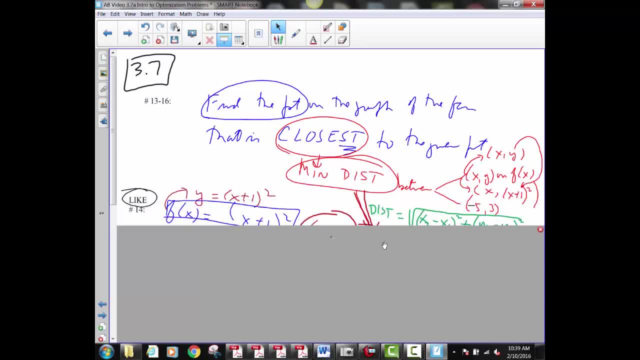 Closest means minimum distance, And the distance between two points is going to be the distance formula. So you've got a point on the curve, some random point x, y, But sorry, in this case this is like number 14.. 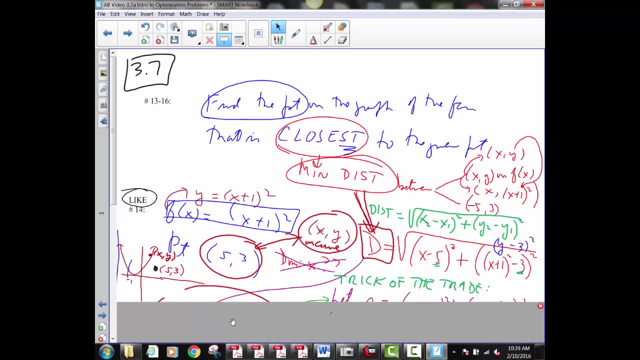 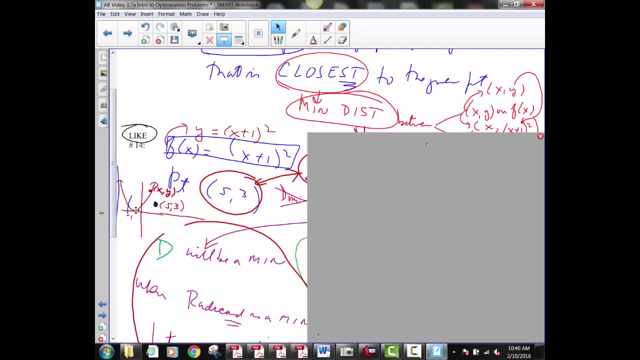 So here's your function and here's your point. So if I draw a picture of this just to not confuse you, so you know that this is a parabola turning up and I moved it to the left one, So I don't know what those blue guys are. 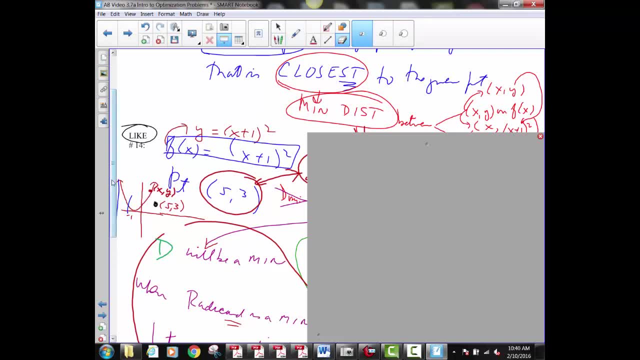 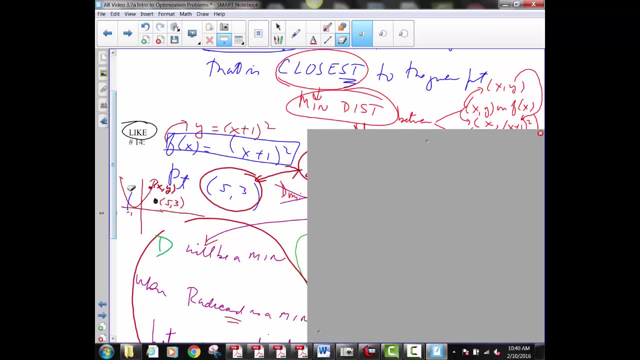 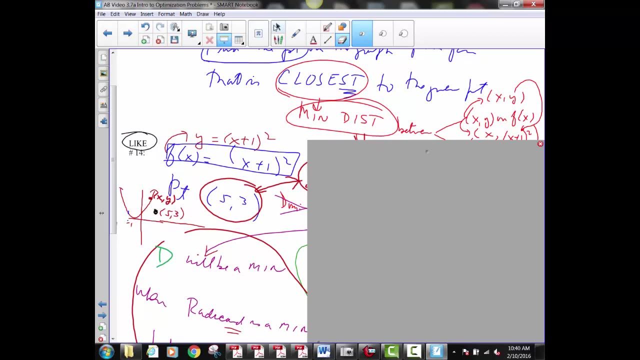 but I don't think I'm going to be able to get rid of them without getting rid of other stuff. And I shall try. Oh not bad, There we go. Yeah, I don't know what that is, Okay, okay, so there's our parabola. 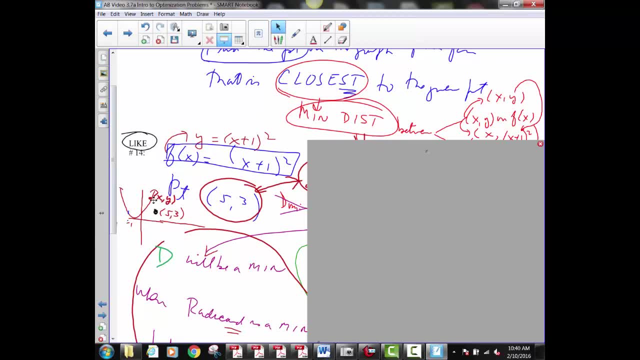 There's a random point on our parabola x, y. that is the closest point on our parabola to the point 5, 3.. So you can see it's not going to be over here. That's way further away. 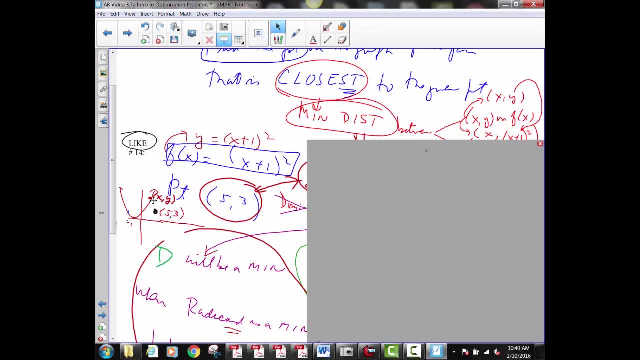 That's further away. I'm just picking some random point- x, y and I'm trying to say that that's the closest point to 5, 3.. But what is that random point? Okay, so the distance will be the distance between the point x, y on the curve. 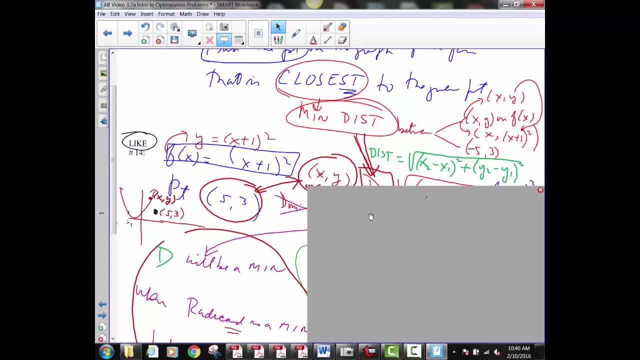 and the point negative. why did I say negative 5, 3?? Oh, it's 5.. Hmm, don't know where that negative came from. Let's delete that. Okay, and the point 5, 3.. Now that point x, y. keep in mind that your y on that graph is actually x plus 1 squared. 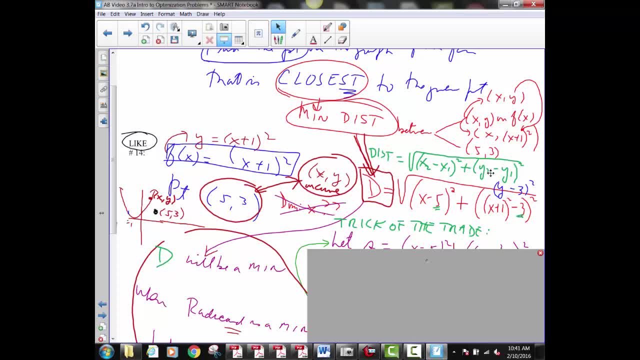 so it's really the point x comma, x plus 1 squared, So you have x2 minus x1.. You get x2 minus x1 squared, which is x minus 5 all squared, and then you have y2 minus y1 all squared. 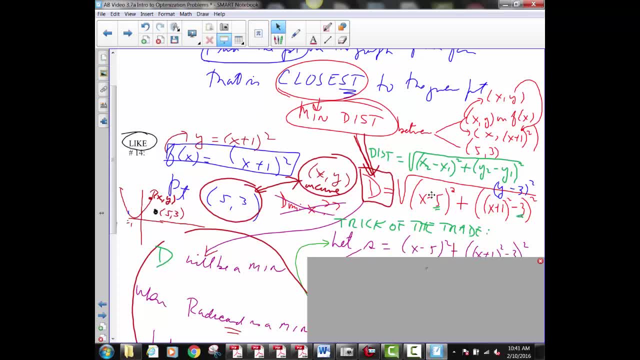 Now the distance is the square root. Now here's a trick of the trade: If you let d equal the square root. if you were doing this by hand, it would not be fun to take the derivative of this because of the square root. 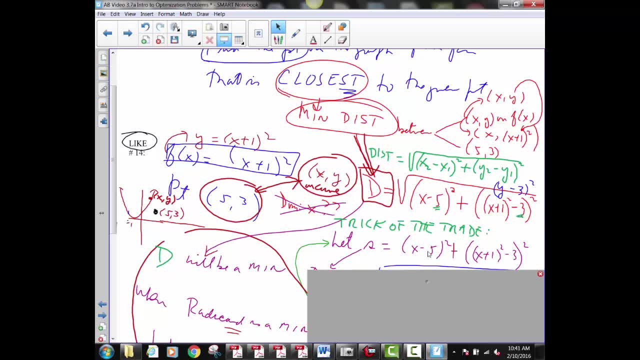 So what they do is they: let s equal the contents of the radical called the radicand, accepting the fact that the square root of something will be a minimum or a maximum when the thing inside it, the radical, is the minimum. 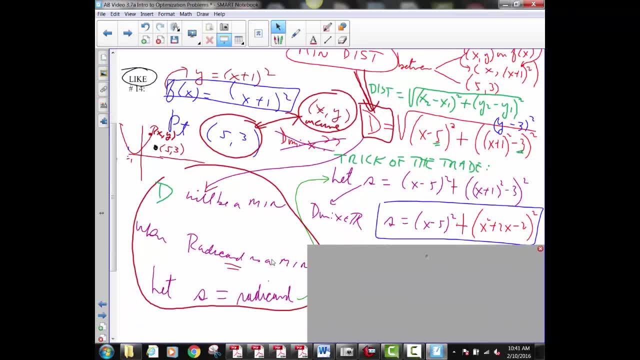 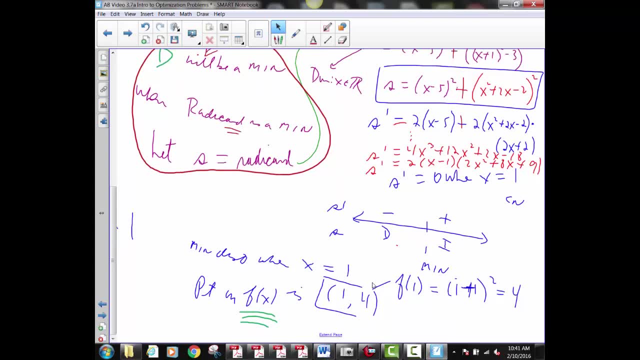 radicand is a min or a max. Okay, the domain would be all real numbers, because we have no idea where this point is going to be. Here's your equation, the derivative, the critical numbers, blah, blah, blah, blah, blah. Okay, you find out there's a min at one. plug one into the original function. 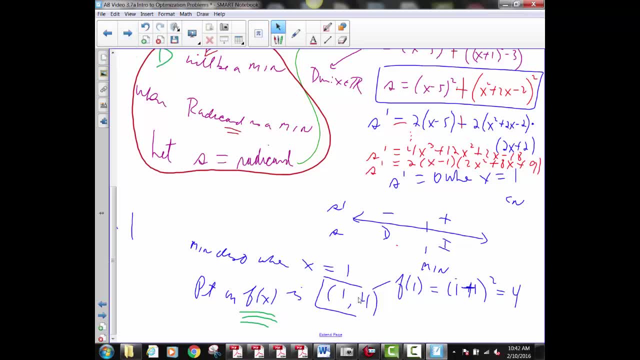 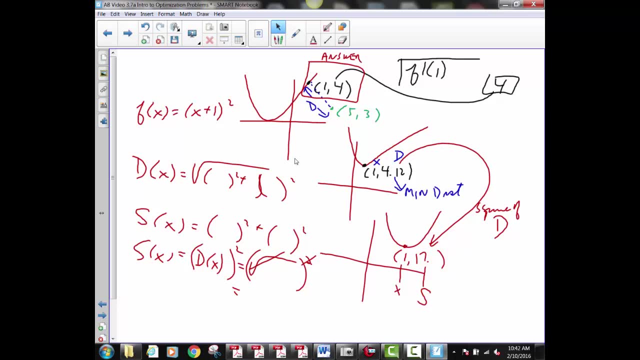 and you'll find that it's the point one, four. So the it happens when x equals one and when y equals four. Now, if you were to graph the derivative, the actual distance equation, okay, on the calculator, you would get this graph and you would get the y coordinate is 4.12,, which is actually. 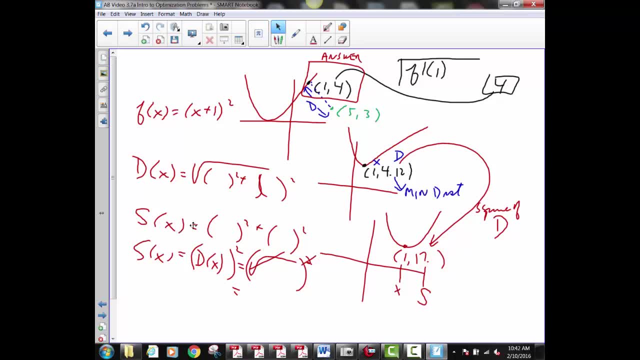 the minimum distance. But if you graph the s version of it without the square root, what you're getting is the value of s, which is 17, as your minimum, and of course, the square root of seven times 17 is your 4.12,. but 17 is not the minimum distance, It's the radicand of the minimum distance. 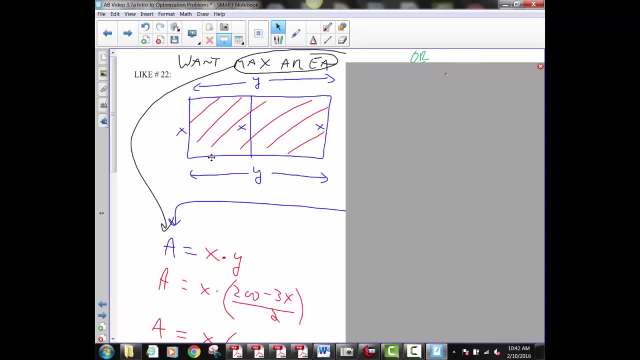 Okay, this is like 22.. You have- these are usually animal pens- and you have a rectangle. you're going to split it somewhere down here, not necessarily in the middle, but you're going to split it so that these animals can't eat these animals. It's always a good plan And so, obviously, being rectangles, 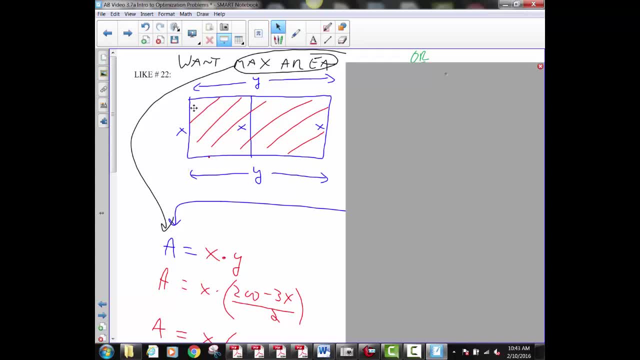 if this is x, this is y, and if this is y, this is y, And so you're going to split it so that this is also x, this is also x. if this is y, this is y, And you want to maximize the area, So you 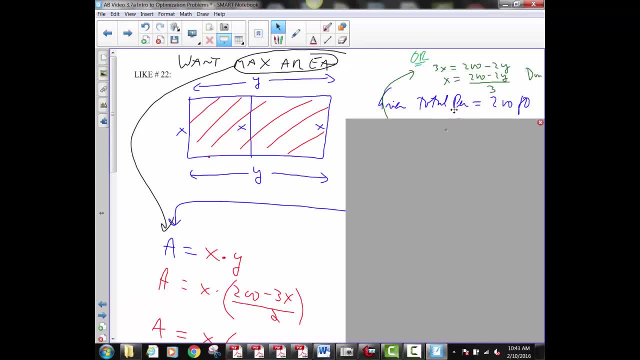 have so much fencing, okay. So you have a total perimeter of 200 feet of fencing. the blue all adds up to 200 feet. Now, of course, we're trying to maximize an area. So the area of the whole thing is y times x, But that's too many variables. I have a x and y, So we come back over here And we